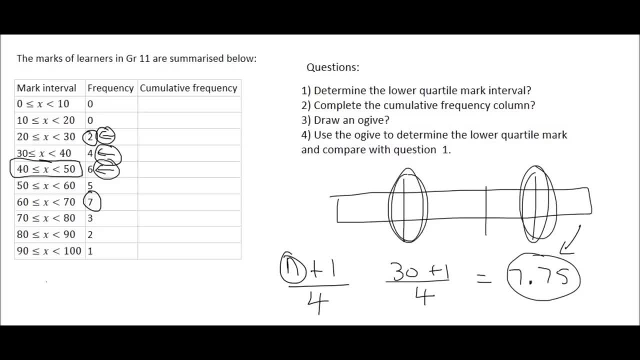 So the 7.75th person would be in that interval. So the answer is going to be: x is bigger than 40, smaller than 50.. Next question says: complete the cumulative frequency column. So cumulative frequency works like this. So because these are a zero in the beginning, we'll just say zero. 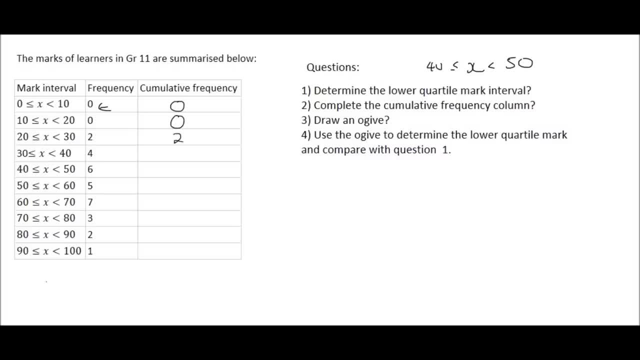 and then the next one's a zero. Now we have a two, so we'll put a two over here. Now we're going to put a six, because, up till that point, how many people have we counted so far? Well, there are six people, And up till this point. well, now we're going to add. 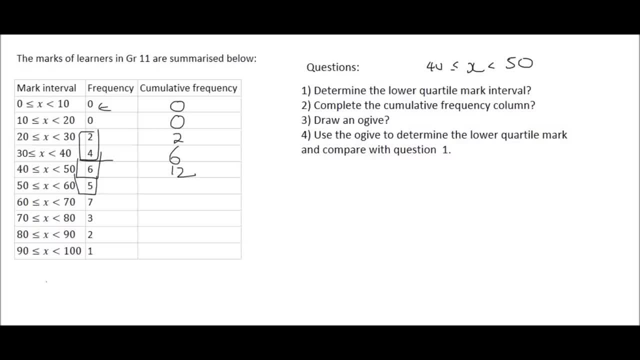 another six, So there's 12 people, And after this five now there's 17 people. After the seven there's 24.. After the three, there's 27.. After the two it's 29.. And after the one. 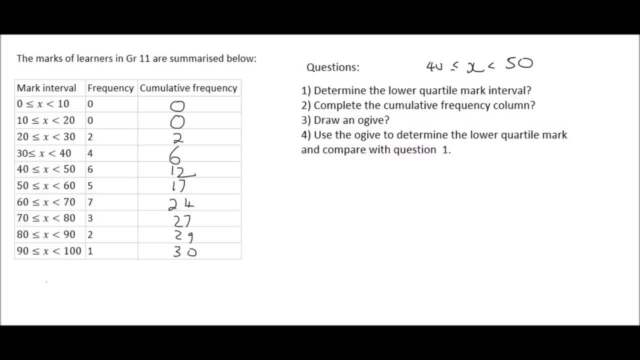 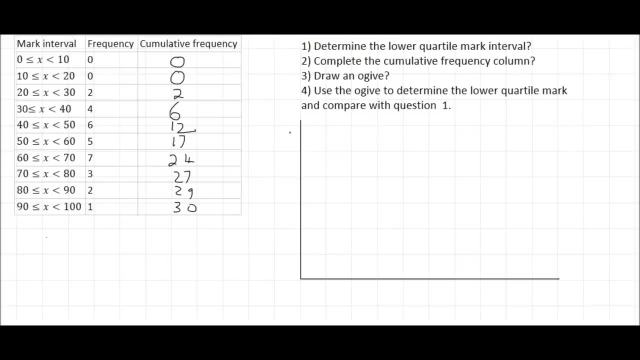 there are 30 people. Cumulative comes from the word accumulate, And accumulate means like gather things together, So when you say cumulative, you're talking about in total. The next question asks us to draw an ogive. With an ogive, your x-axis is always going. 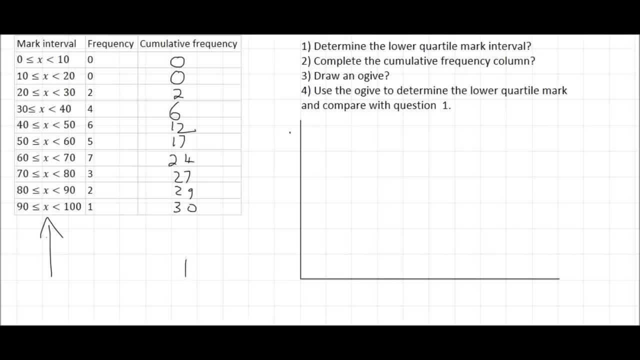 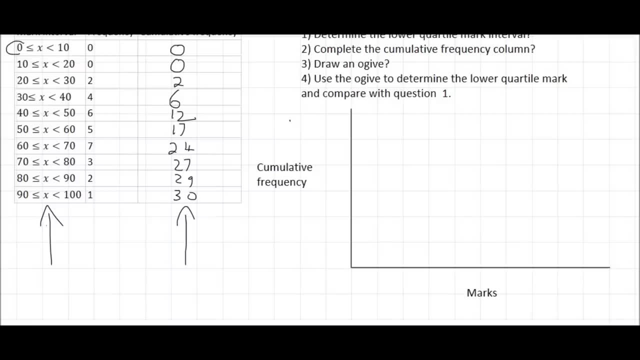 to come from this column over here And your y-axis is always going to be the cumulative frequency, Then what you want to do is the following: This number over here that you always see in the beginning of your mark intervals, always let that be your first value over here. 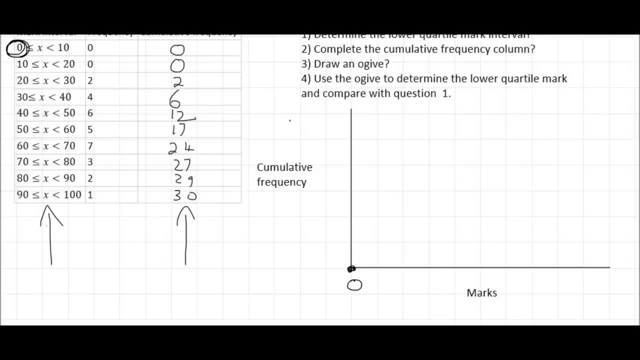 Okay, so in this case it's a zero. Then what you want to do is you want to use these values on the edges for the next parts. You don't want to use the midpoint values when you're doing an ogive like that over there, And then you can just find a. 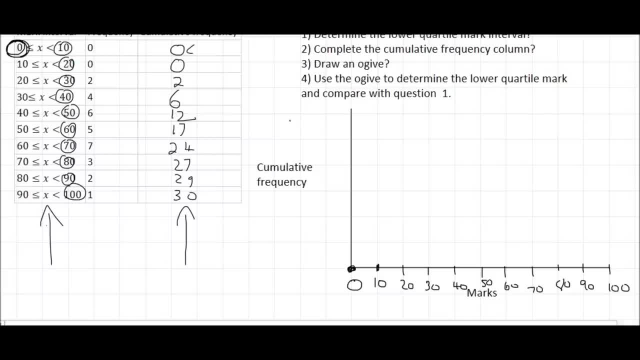 suitable scale for your cumulative. Well, we know that the cumulative is starting at zero, So we can put another little zero over here, And it's going all the way up to 30, like that over there, And now you simply go plot the points. So for the first one it's going to be 10.. And also 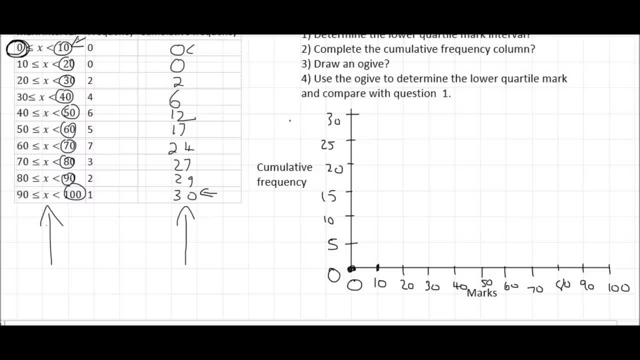 the first one, it's just going to be this: 10 over here and zero, So that's just over there. The next one is going to be 20 and zero, So that's still over there. Then it's going to be the number 30. So we always use the end value. 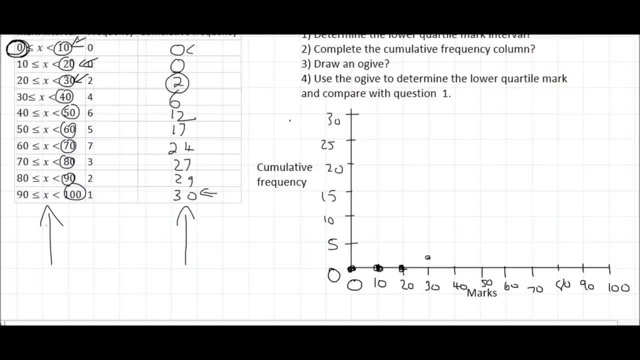 and two, So 30 and two- it's approximately over there- Then the number 40 and six, which is approximately there, Then it's the number 50 and 12. And then you just go ahead and plot everything else. Once the dots are complete, you can just. 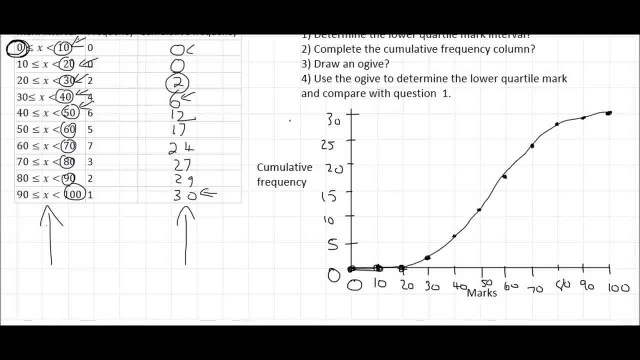 try to draw a nice neat curve through the dots And it will always form that kind of S shape like that. Okay, it'll never go downwards. Why? Because we're using these cumulative frequency numbers and those numbers always get bigger and bigger. And the last question says: 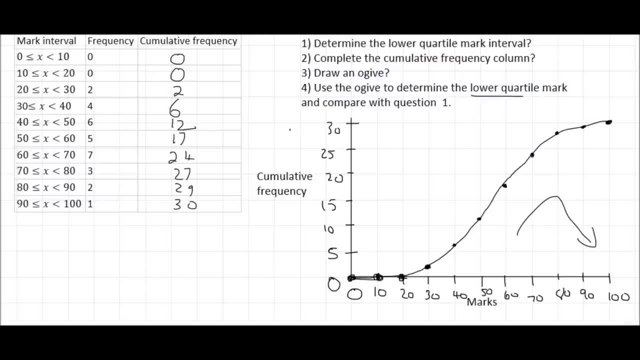 use the ogive to determine the lower quartile mark and compare with question one. So in question one we read the quartile mark, the lower quartile mark from the table. the interval of that was the 40 to 50.. Okay, so we said that x was bigger than 40 and smaller than 50.. 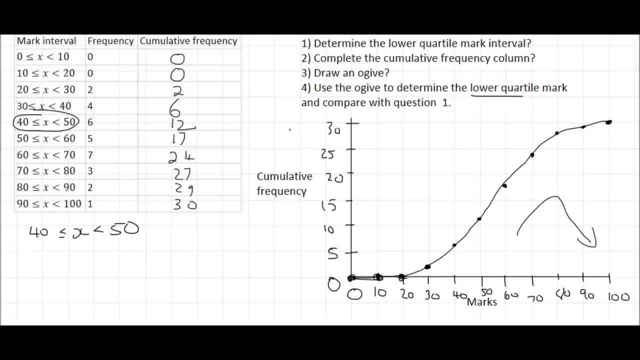 Now we're going to determine the lower quartile mark on the ogive, because using the table is not very accurate because it's. we know that the mark is somewhere in between here, But when you use an ogive you can actually get even closer. Let's see how that works. So it says: use the ogive to. 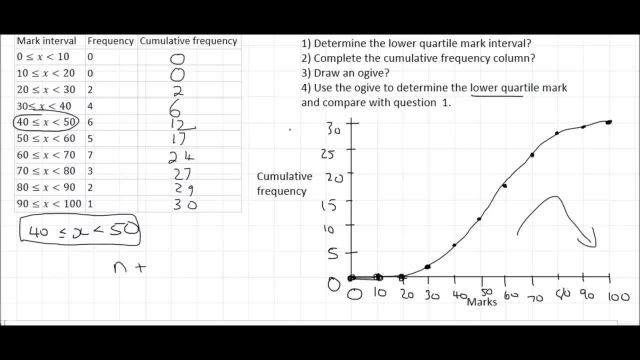 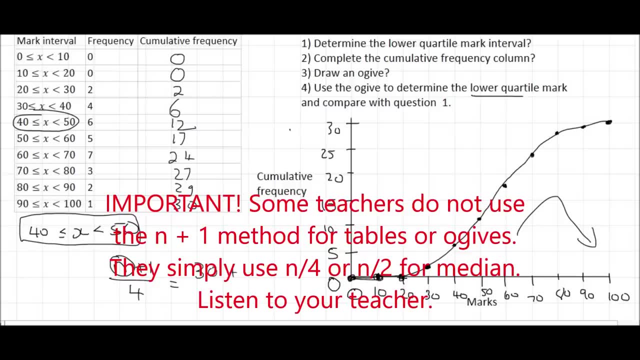 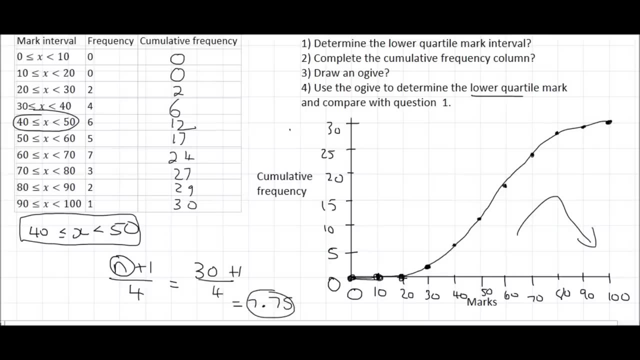 determine the lower quartile mark. So the lower quartile is always n plus 1 over 4.. n is always the number of values that you have, And in this case we have 30 people, So it's 30 plus 1 over 4, which is 7.75.. So we have to find the 7.75th person. Would you find the? 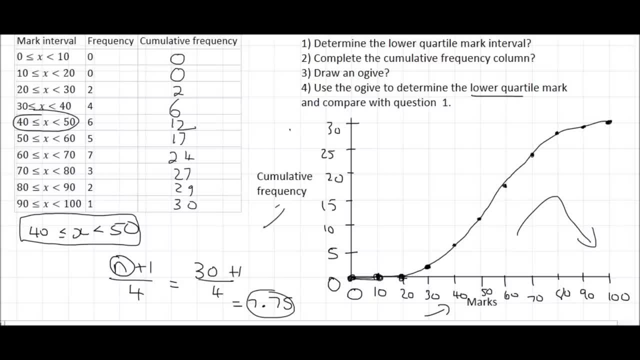 7.75th person looking at the marks or looking at the cumulative frequency, Because, remember, the cumulative frequency is the number of people you have counted so far. So, for example, over here you've counted two people, Then over here you've counted six people in total, because there were two people here and four people. 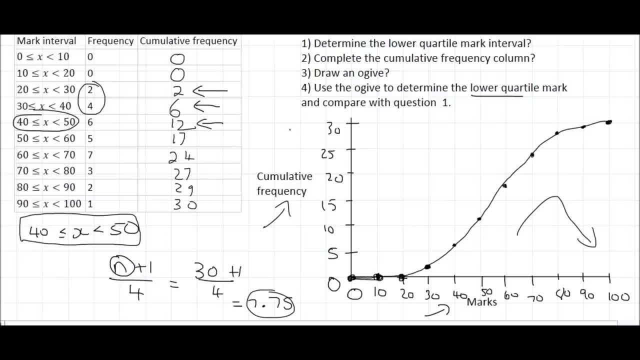 over there. Then for the third one, you've counted 12 people in total, So the cumulative frequency is the number of people you have counted in total so far. So we need to go find the 7.75th person. So that'll be somewhere over here. You would then draw a line going across and then you would go down.